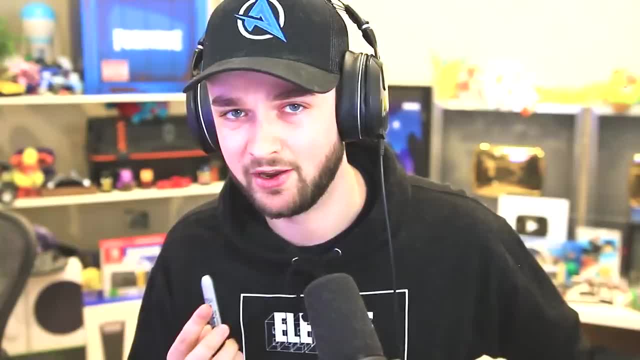 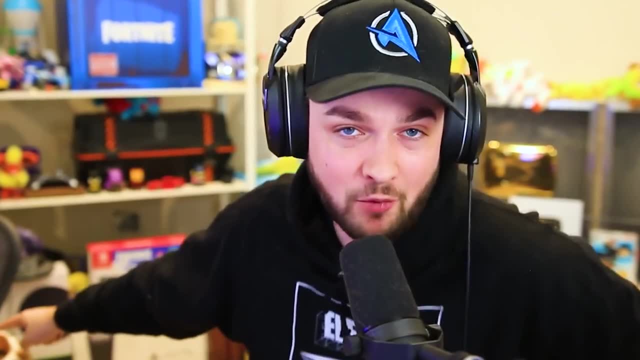 Today we're going to be checking out some incredible TikTok magic and exposing exactly how the magic tricks are done. Stick around to the end to see some crazy bonus magic. and if you're watching right now and you want to give Eevee one pat on the head, 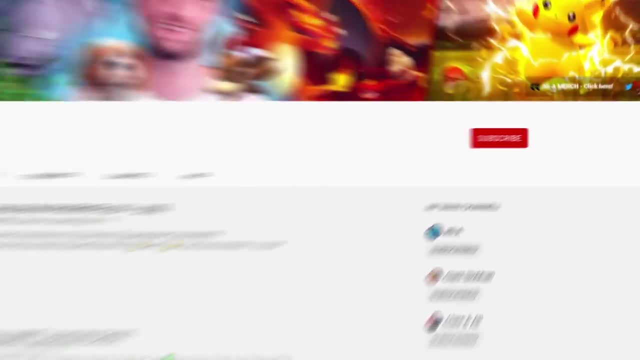 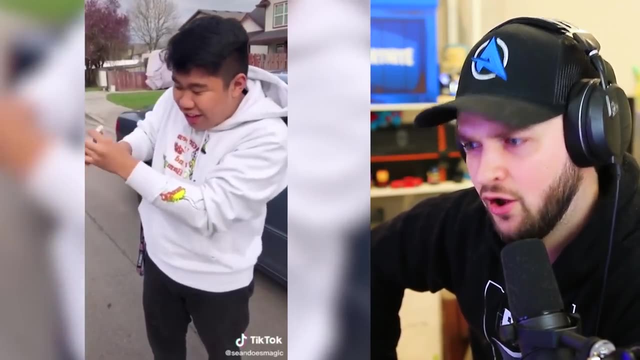 hit the like button right now and don't forget to subscribe. Teach me a magic trick. I got you. I'm about to teach you how to take any red deck of cards. give it a little rub, Okay, And it literally changes to a blue deck. 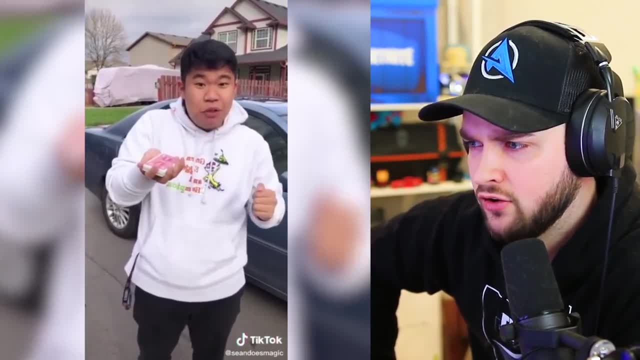 What? This is actually really easy. All you need is the right card. Take that place on top of the blue deck of cards. All you're doing is you're pushing that card forward, using your palm to bring the card back and placing that-. 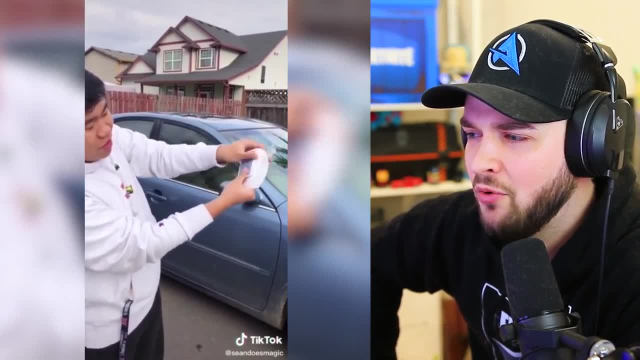 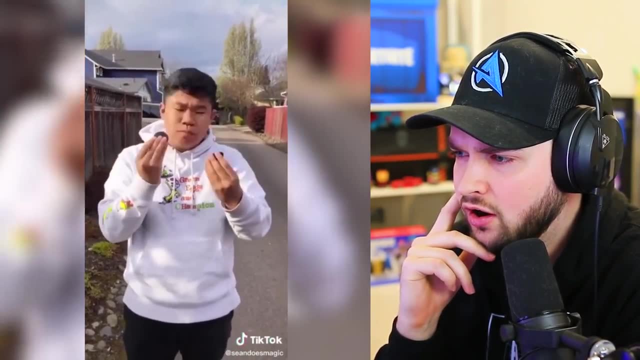 Oh, All at once it looks like it changes- I wondered where it went. He's so clever, I got you. I'm about to show you how to take any Oreo, lick all the frosting off and literally get it to refill, just like that. 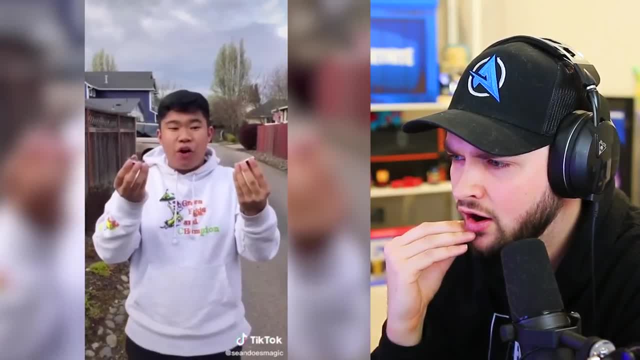 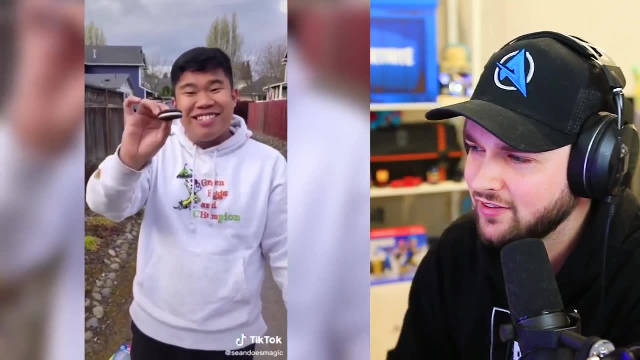 What To do this? it's actually really easy. All you need to do is eat one half of the frosting, and one side is going to have no filling and the other side- Oh, Oh, Oh. All magic tricks that we can pull off. This Sean guy is incredible. 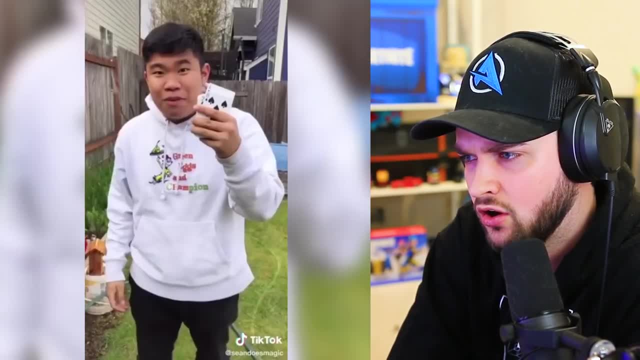 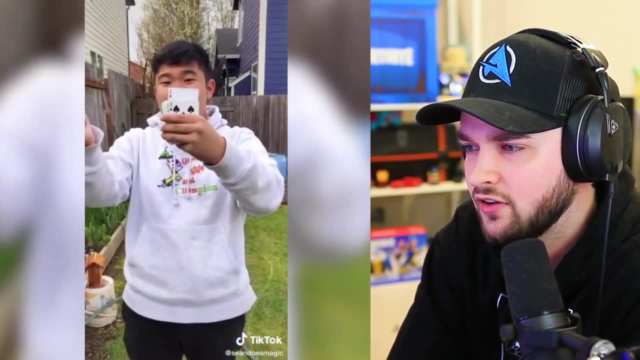 I'm about to teach you how to take any deck of cards and magically make a card pop. Whoa. To do this, all you need is two cards. All you gotta do is- A what A rubber band to it. This acts as a spring, and any card in between it will magically pop out. 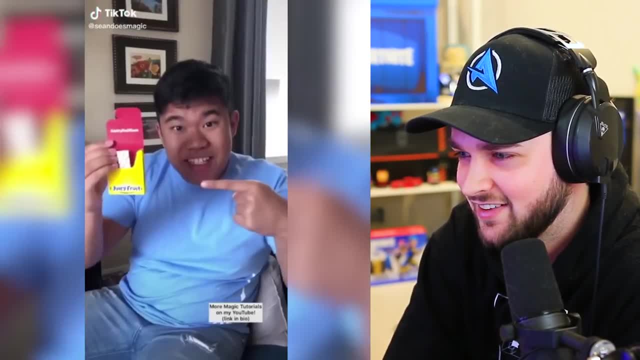 What, Sean, Sean, Sean, What's up? Teach me a magic trick. I got you. I'm about to teach you how to take an empty pack of gum. snap your fingers- Shake. See that Suddenly it's a full pack of gum. 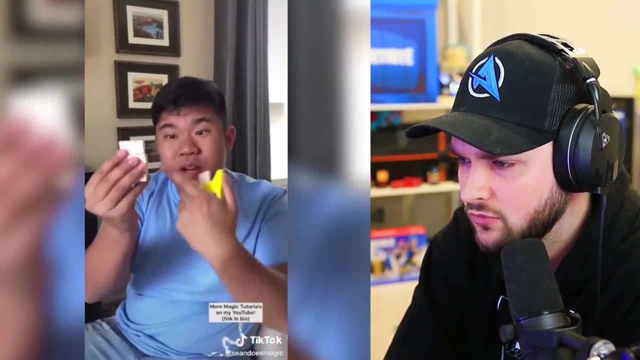 This guy- How does he do it? Teach me A bunch of gum cut in half stuck together. Put that inside there And all you're doing is you're tilting it upside down so that they all fall out. Ah. 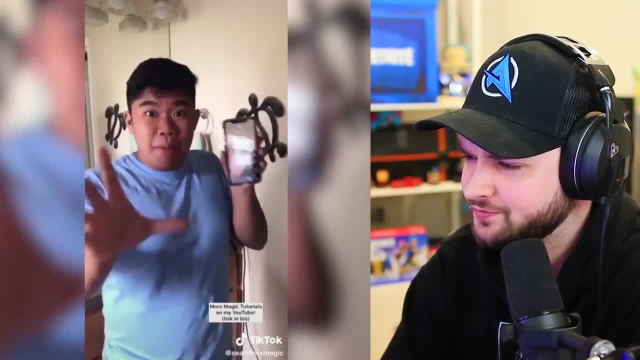 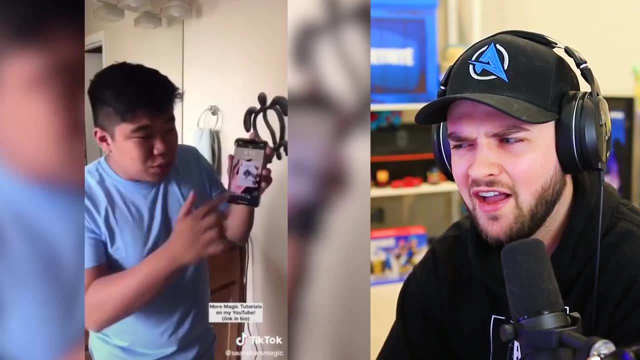 Bam. The answer's always so simple, but it works so well. I'm about to show you how you can take any wallpaper- like the Ace of Spades, just like that, and magically change it. To do this, what you need is a screenshot of any wallpaper- 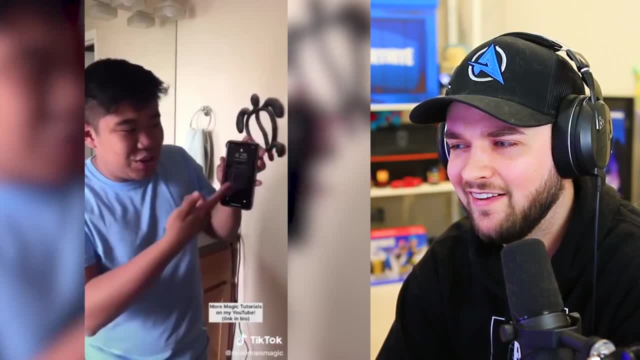 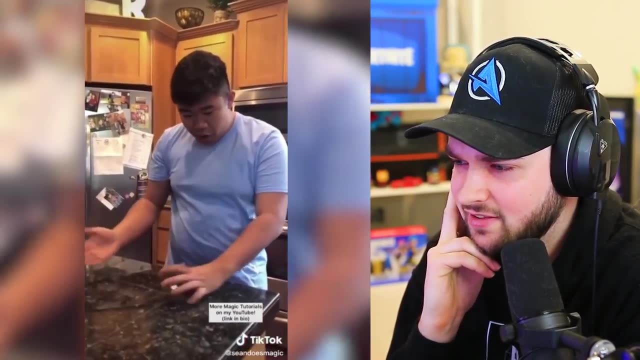 Oh, And literally all you're doing is turning off the phone and turning it back on and it will show the actual-. That's so smart. Touch a shot. I love it. Do a magic trick, I got you. I'm about to show you how to take any AirPod and literally-. 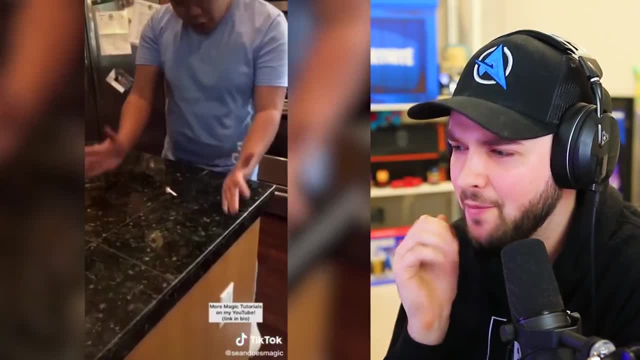 To do this, what you need is a table. Don't steal my AirPods. It looks like you're picking up the AirPod, but in reality, what you're really doing is you're just dropping it to the ground, Ah-haaah. 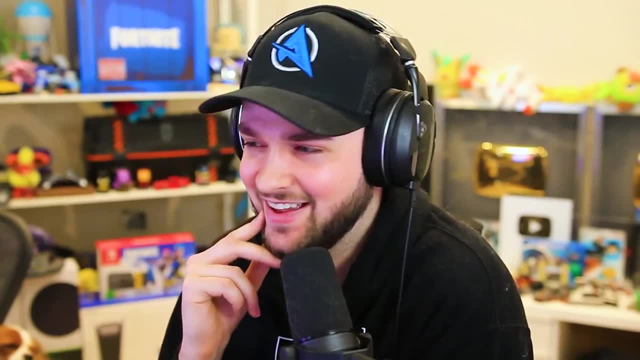 You can make it look like it really vanished. That's a good idea. So teach me a magic trick. What's he doing? I got you. I'm about to teach you how to take a pencil and make it go right through your hand. 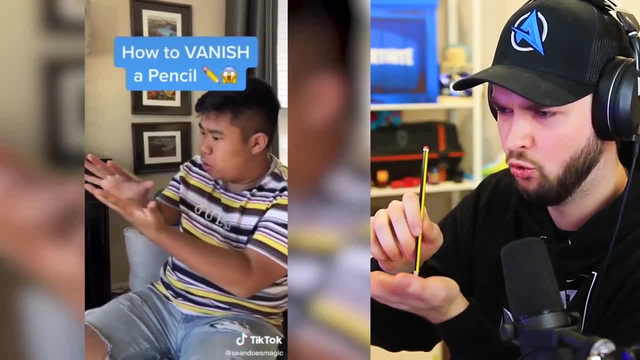 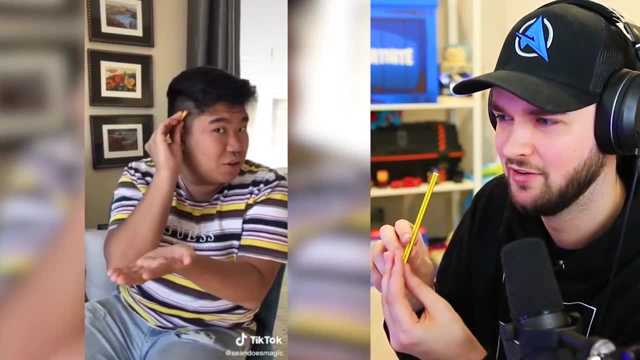 I've got one here On the count of three, Three, two, one. Oh my- that looks painful. This trick uses misdirection. All you're gonna do is, as you count down- One, two- On the third one, you put it behind your ear- 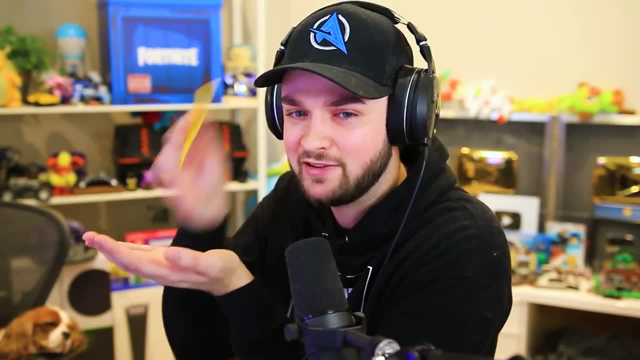 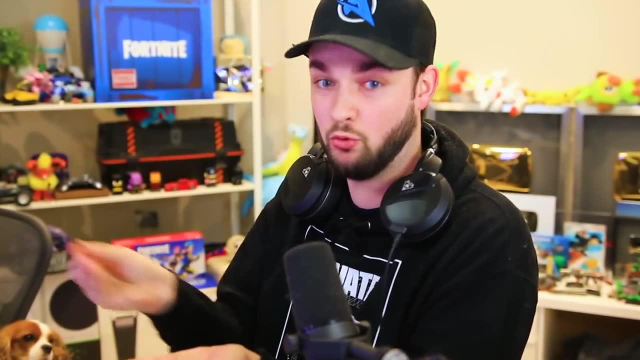 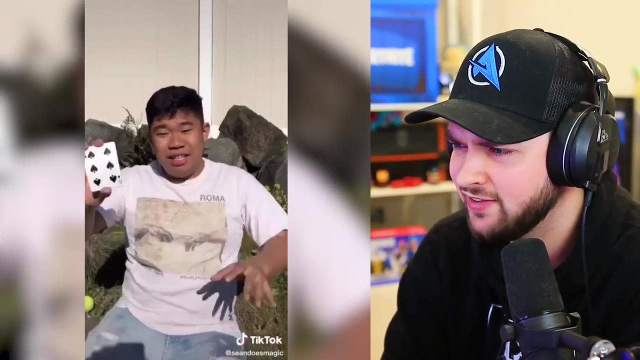 What Can I do it, Guys? I'm about to make this pencil disappear. That did not work at all. Ooh, I'm a magician. now I'm about to teach you how to- Barf cards from your mouth. What? 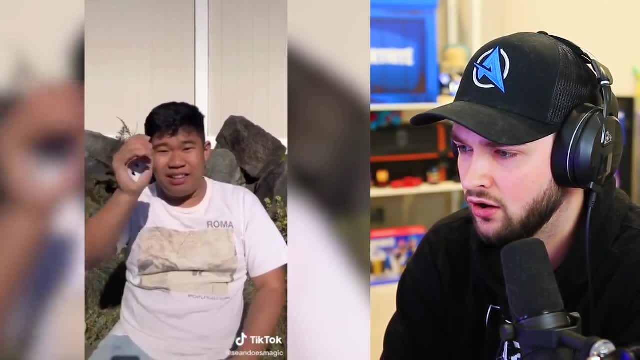 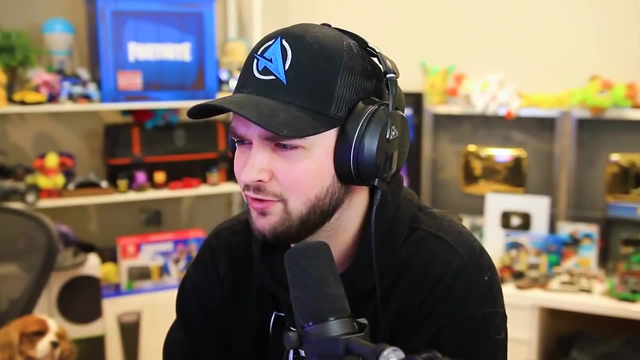 This one's really easy. All you need is a small packet of cards. Have it hidden in your hand like this, and you're just gonna- Peel all the cards from your mouth Altogether. it looks like this. It looks so good, though. 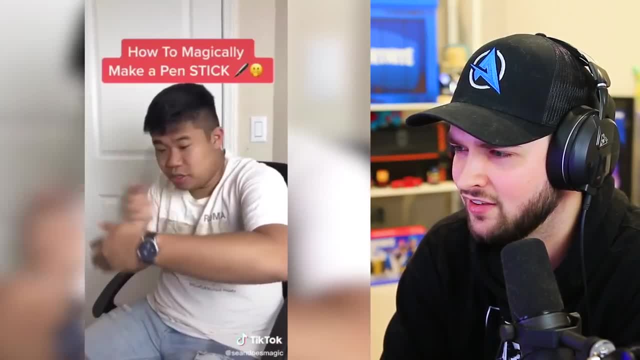 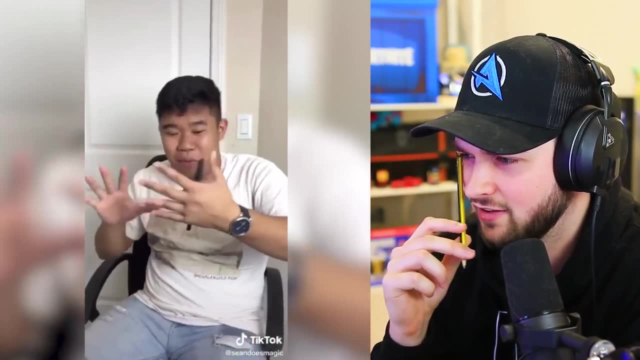 I'm about to teach you how to take a pen- Get it, Get static electricity and get it to literally stick to your hand- And no, I'm not using my other hand. Okay, The secret to this is really simple: All you need is a watch or a bracelet. 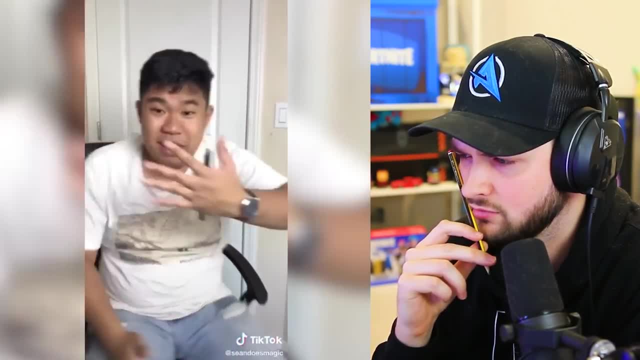 Place a pencil right inside here. All you gotta do is place it right there And then, bam, it looks like the pen is sticking. I can't do that. I don't have a watch. That's sick. I'm about to teach you how to take any water bottle-. 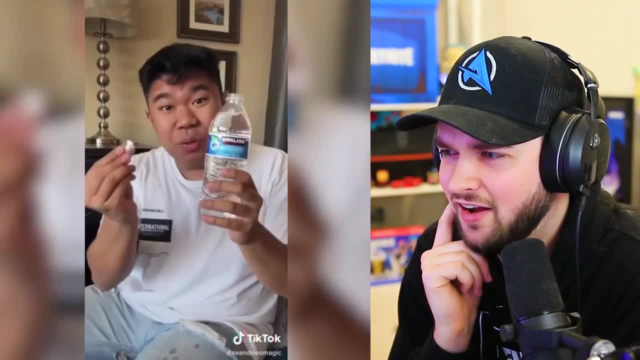 And get it to magically stay up in place. Wait, Whoa, This is really easy. All you need is a little plastic disc like this. That seems dangerous. Yeah, And what you do is, as you turn it over, you're just gonna place it on top of that little plastic disc. 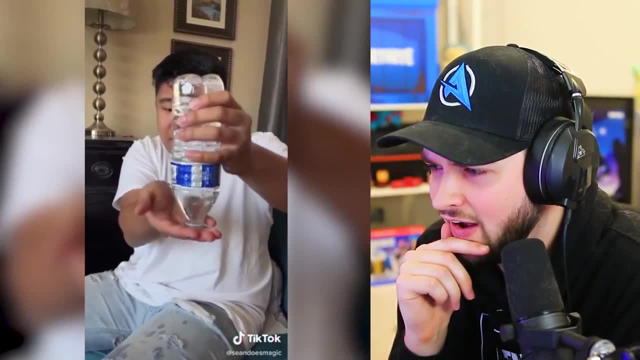 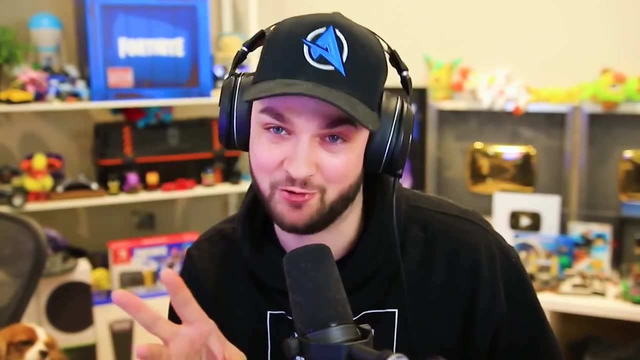 And what you do is, as you turn it over, you're just gonna place it on top of that little plastic disc And it'll hold the water in place, just like that. That seems like if you do that wrong, there's a lot of water going everywhere. 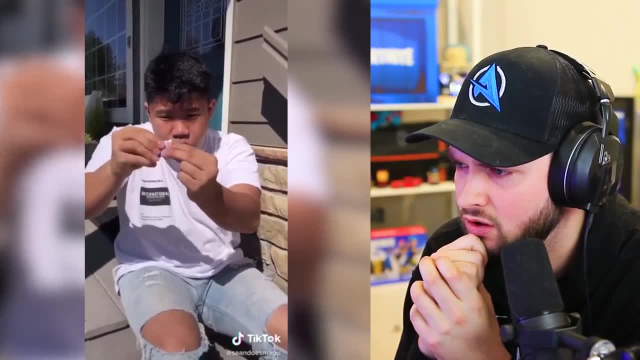 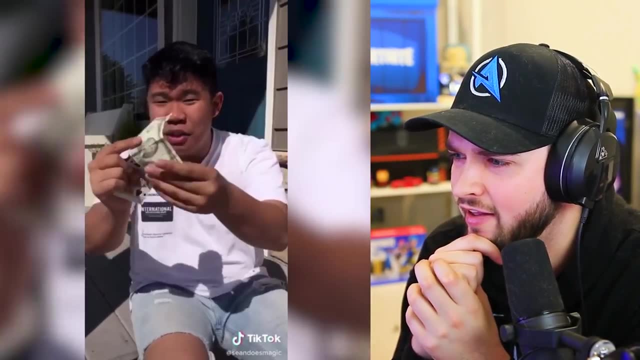 I got you. I'm about to teach you how to take any card, fold it up and change it right into a two dollar bill. What, Whoa? To do this, you're gonna need a card and a dollar bill. Take the bill and fold it into a card-like shape, like so. 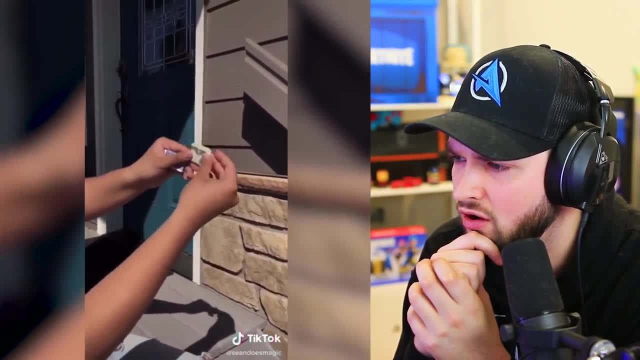 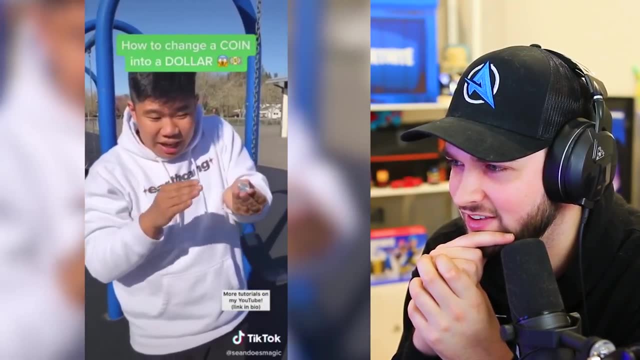 As you fold, you're gonna switch the two pieces. Ah, And the card looks like this. Just like that Clever. So teach me a magic trick. I got you. I'm about to teach you how to take any quarter wave and change it right into a dollar bill. 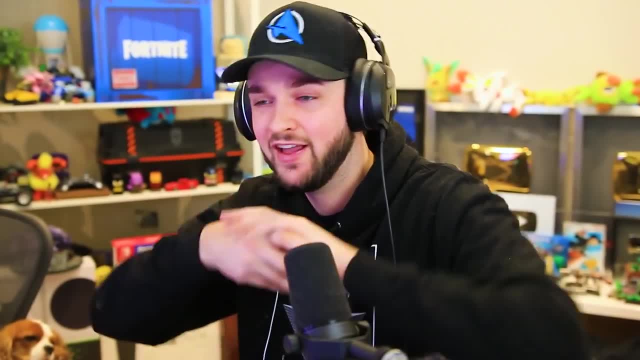 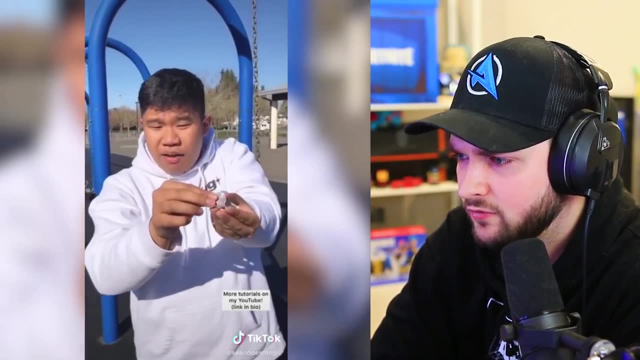 What, Yo? I wish I could do that in real life. Here's a quarter. Here's more money. I'm gonna create infinite money for us all, Really easy. All you need is a folded bill like this. What you wanna do is hold it right here and have the quarter hide the bill from the back. 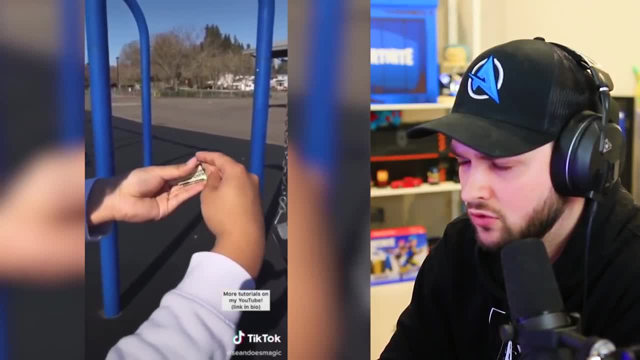 And all you're doing is, as you're waving over, you're gonna push the coin down into your hand and then you're gonna bring this bill forward. All in all, it looks like this: You grab it. Oh, it's like sleight of hand. 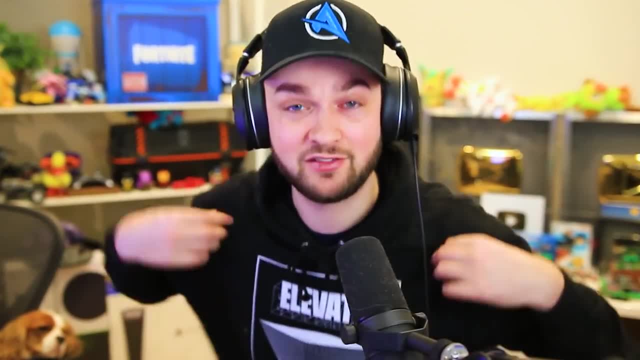 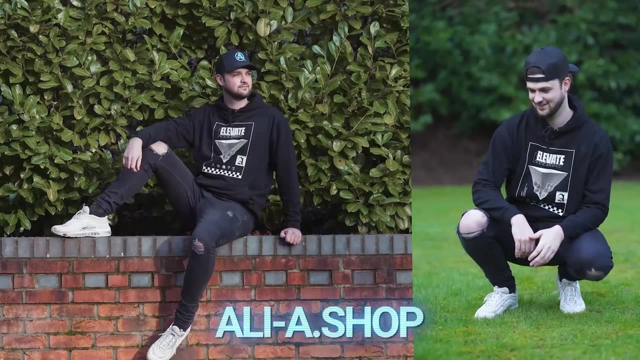 The bill appears So smart, I've got an awesome magic trick for you guys. You see the hoodie I've got on right now. Well, you can have it on as well, with the new Elevate merch launch dropping tomorrow at Allieshop. 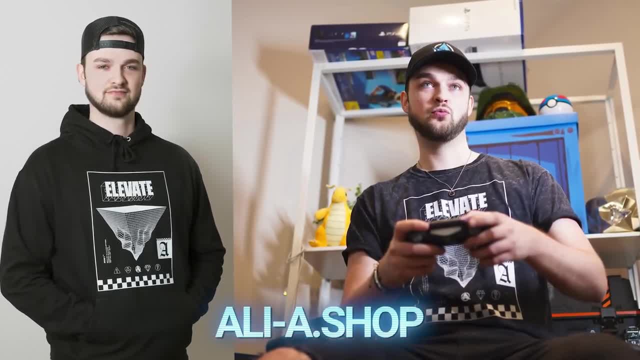 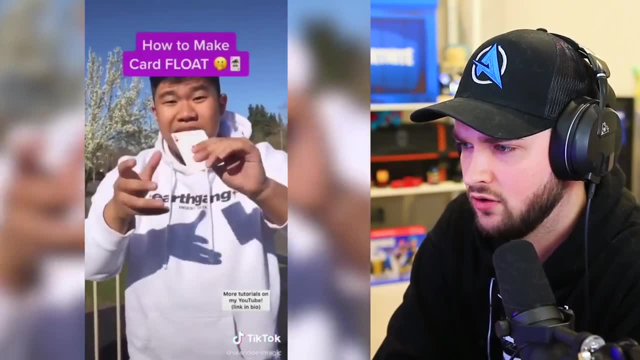 with an epic new Elevate design on t-shirts and hoodies. Check out Allieshop Thursday, the 28th of January. Don't miss out to get the exact same hoodie I'm wearing now. I'm about to teach you how to take any card and make it look like it's whoa floating. 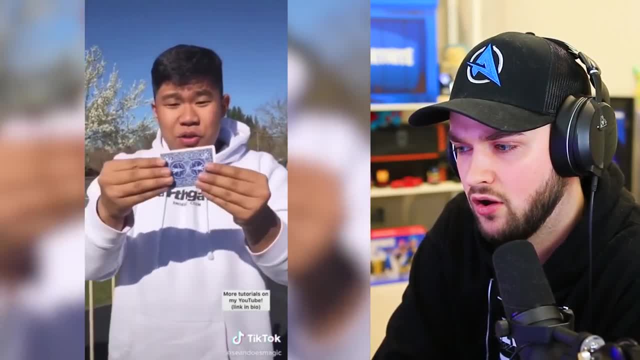 Floating. To do this is actually really easy. All you need is a card And all you're doing is you're using your thumbs right here, Cover it up And you move it up and down. It looks like it's floating. Guys, you ready for this? 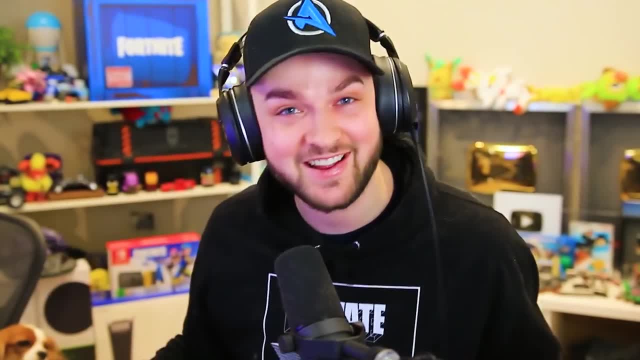 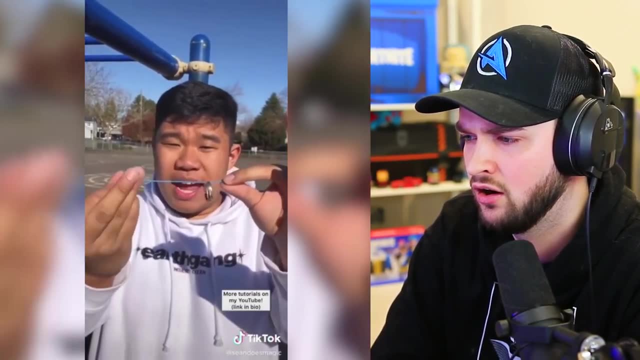 Whoa Yo, it actually looks sick. I did it. What the It's defying gravity. To do this, what you need is a broken rubber band. Place the ring inside the rubber band. Have it closer to one end. 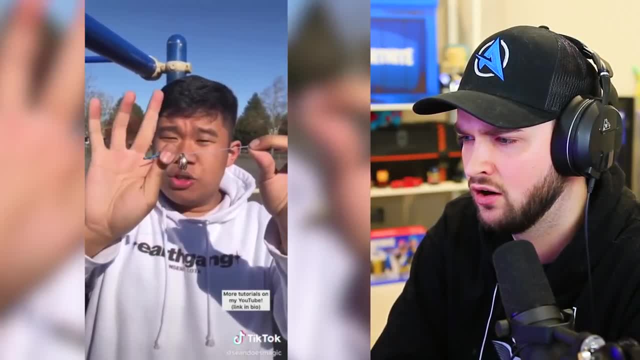 And then grab the rest of the rubber band in your other hand. Stretch the rubber band out And all you're gonna do is release that extra part And it will slowly make the ring rise. Ah clever, Teach me a magic trick. 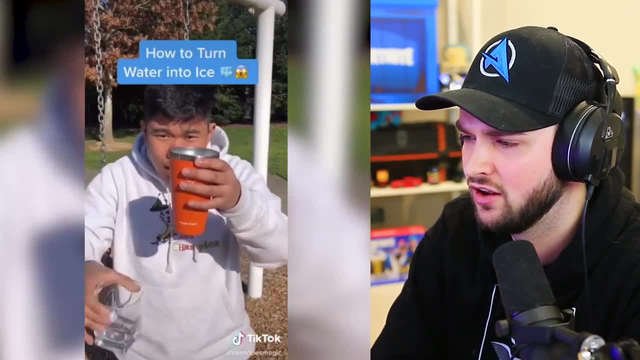 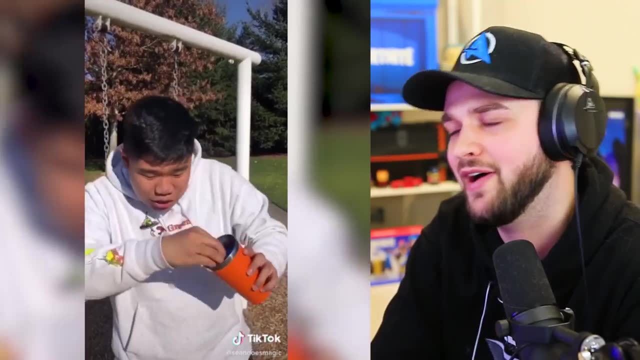 I got you. I'm about to teach you how to take any amount of water, Pour into a cup, Mix it around a little bit And then, bam Ice. This is actually really easy. All you need is a sponge, Oh sponge. 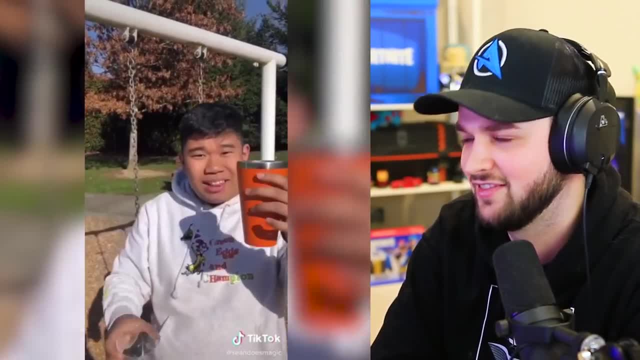 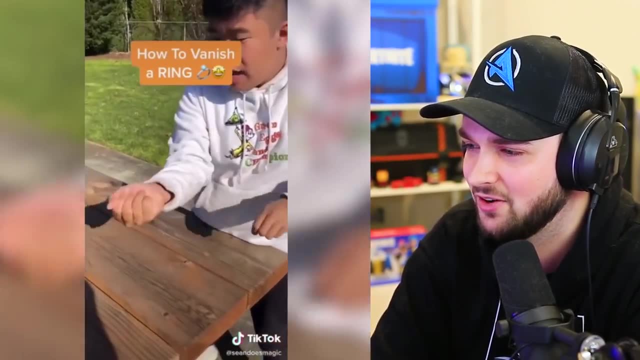 Clever And that sponge is gonna absorb all of that liquid. It's gonna look like it turns into ice Clever Big brain. I got you. I'm about to teach you how to take any ring. Oh my gosh. 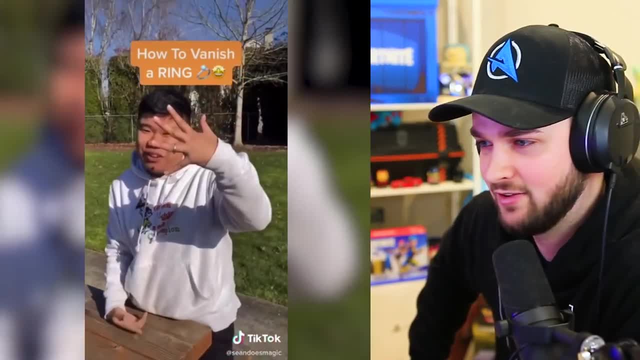 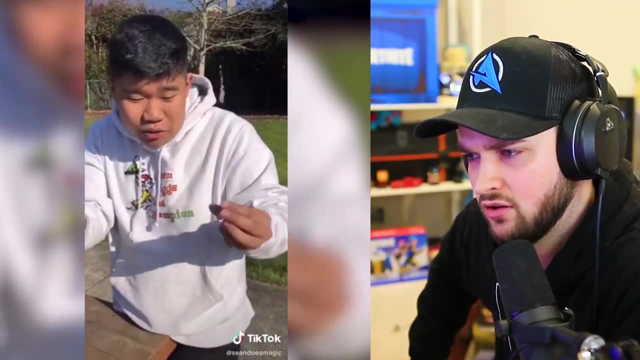 Three, two, one. I don't trust this guy with my money or rings. No way, This one's really easy. What you're gonna do is you're gonna pretend to grab the ring, But really you're dropping it, And while their eyes are in this hand, what you're doing with the other hand is you're. 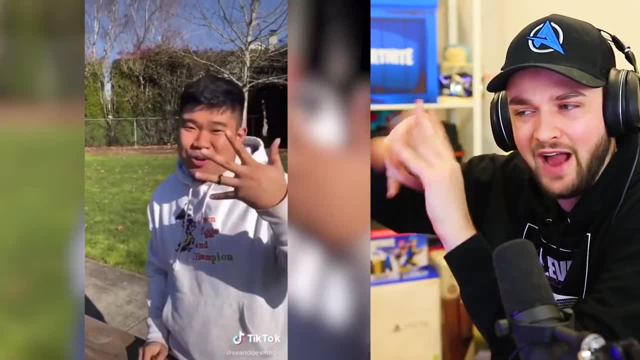 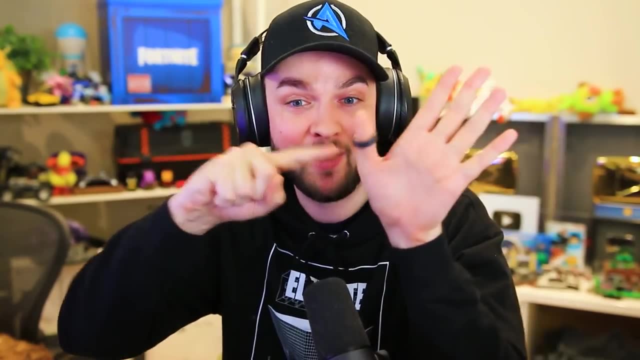 placing the ring. Ah, It's all magic Magicry with the hands. Guys, are you ready for my own magic trick? I've got a ring here, I'm gonna make it disappear. And you ready for this? Bam, It's on my thumb. 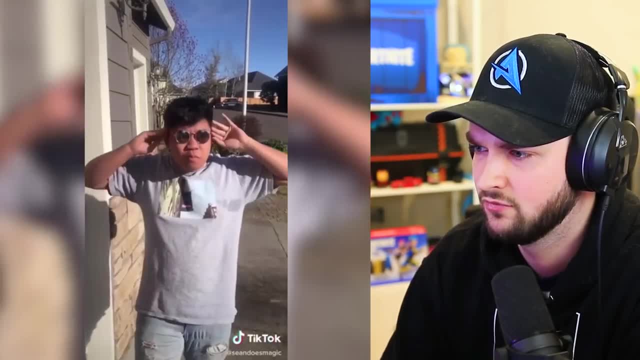 Did it work? Did I put it off? I'm about to teach you how to magically put on glasses. What? This trick's pretty easy. This one's sick. What you want to do is cover the lenses with your two hands, like this. 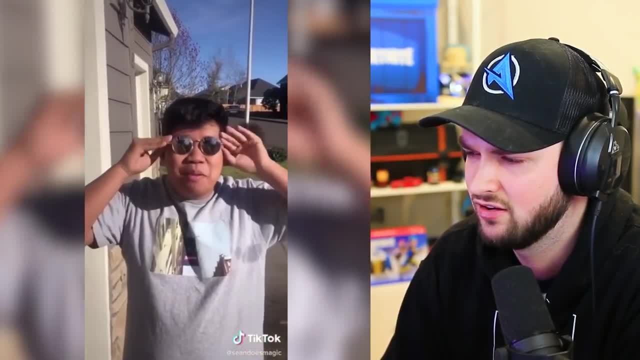 Make sure that you're not flashing the top And then just slowly put them on And bam, You got glasses. I'm about to teach you how to vanish a Sharpie by just grabbing it And then make it reappear, Okay. 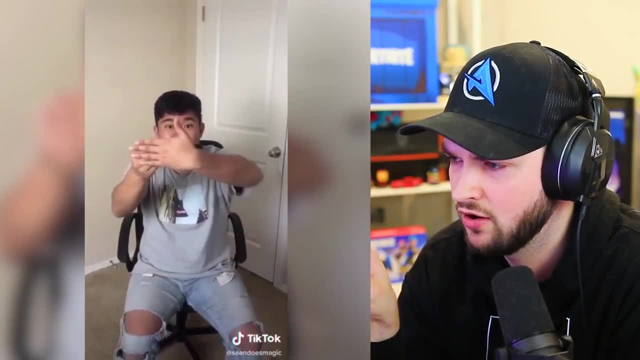 I want to try it some too. All I'm doing is I'm bringing the Sharpie behind my hand like that, While also covering it All together. it looks like this: Vanish Reappear Guys, we're gonna make it disappear. 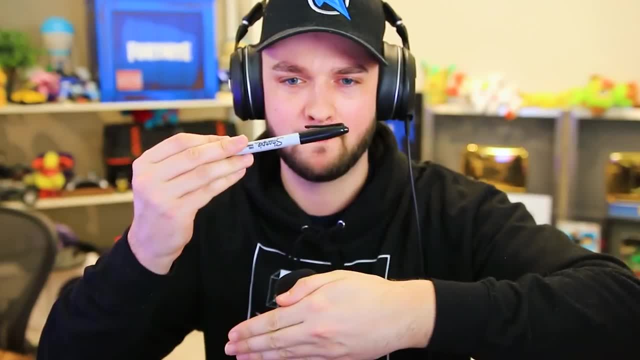 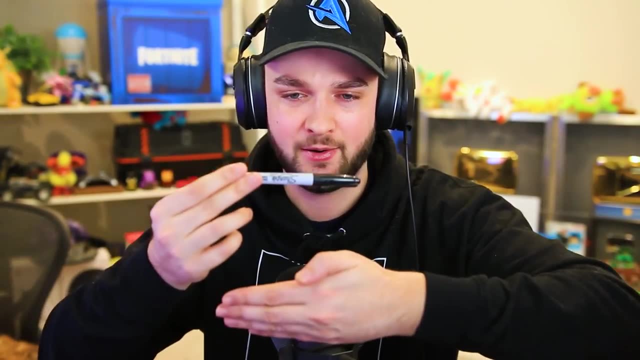 You ready? Here it is There. Wait, wait, wait. I'm new. I'm new to this magic stuff. All right, Give me a break. It goes, It comes back. Woo, I'm about to teach you how to take any AirPod. 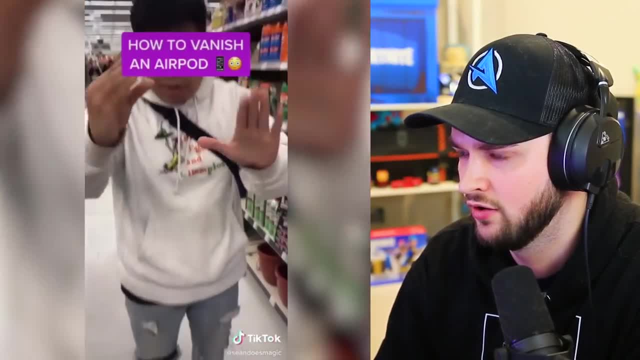 Put it in one hand And make it vanish. Whoa, This one's really easy. What you're gonna do is you're gonna have the AirPod in one hand, And what you're gonna do is you're gonna pretend to place it in here. 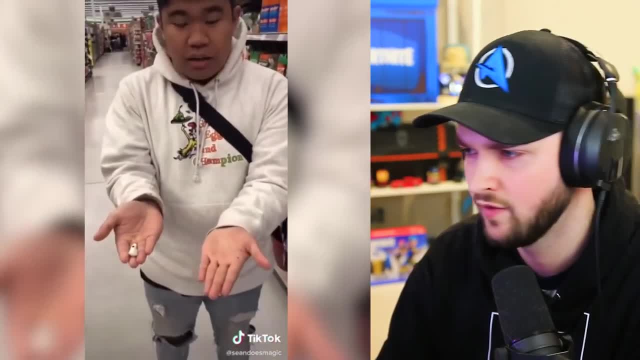 But your thumb is gonna hold the AirPod in one hand And then you're gonna put it back, And then you're gonna put it back, You're gonna pretend to grab it, The AirPod's still in this hand, And then you make it vanish. 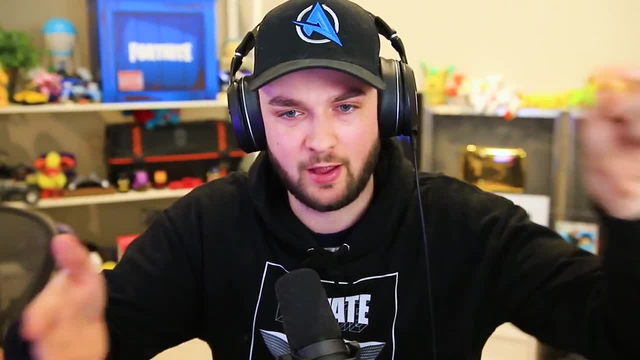 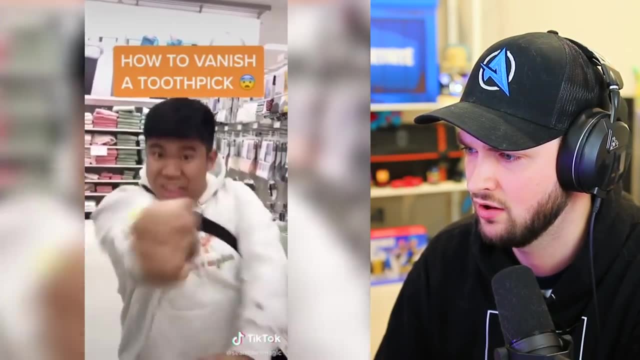 Oh guys, I'm gonna make this control freak disappear Magic. I'm about to show you how to take any toothpick, Make it vanish And then reappear What It's actually a waste of time. Where'd it go? 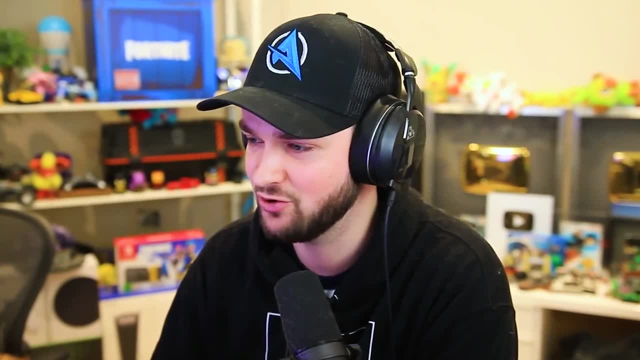 Oh, tape. I'm gonna have to pull these off and impress people with my new found magic trick. Thank you, Shaun. I'm about to show you how to take any Sharpie, Put it up your nose And out your mouth. 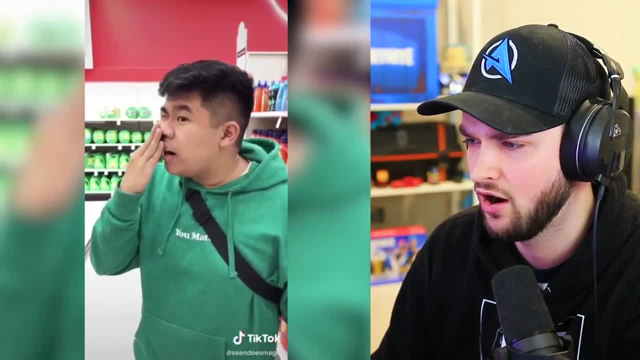 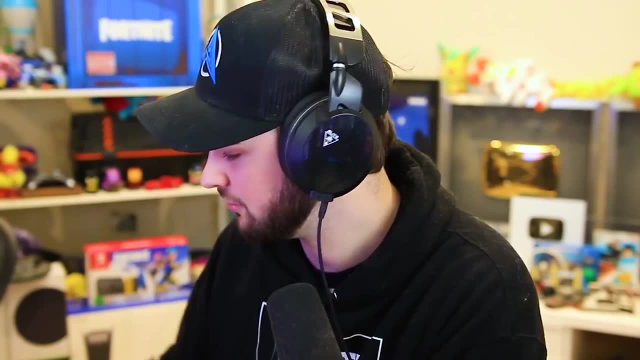 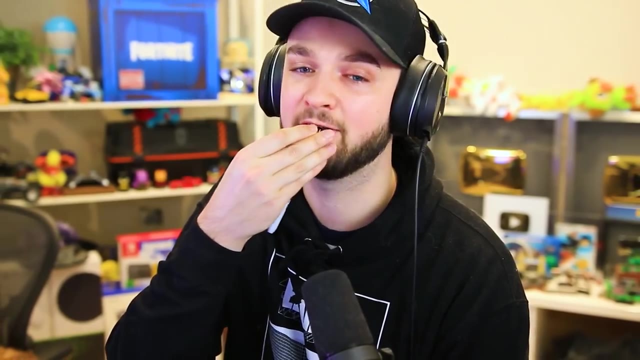 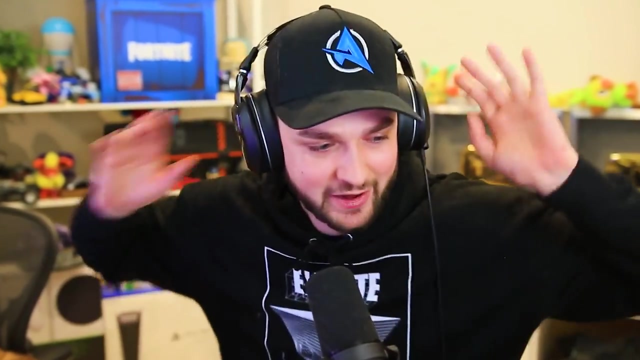 No, It's really easy. This looks so disgusting. Move your hand up. I Think I can do this one. guys, I'm gonna make this sharpie disappear up my nose And up my mouth. Guys, I'm gonna make this sharpie Grab my mouth. Was that okay? I like pulling any of these off. Let me know, Oh, what would that come from?